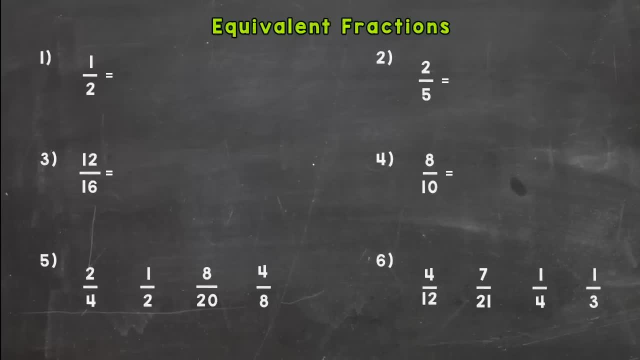 for overall number sense for everyday life. So there's a couple rules we are going to need to follow, with one main big rule that we'll get into once we start, number 1.. But for number 1,, 2,, 3, and 4, those top four, there we are going to. 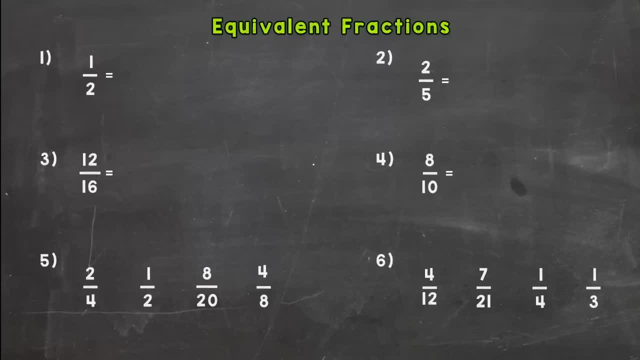 find two equivalent fractions for each two, And then 5 and 6, we will go over what we'll do for those when we get there And after this video. this is the instructional video. the mastery check will be the exact same thing as this. 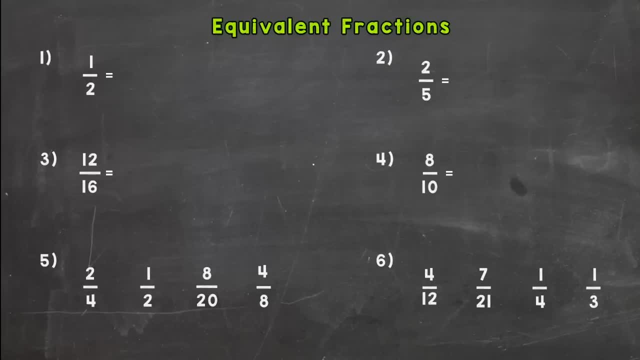 You'll find two equivalent fractions for for each, and then you'll have a five and a six. So let's hop into number one here and we have one half. So our main big rule for equivalent fractions is: whatever you do to the numerator you need to do. 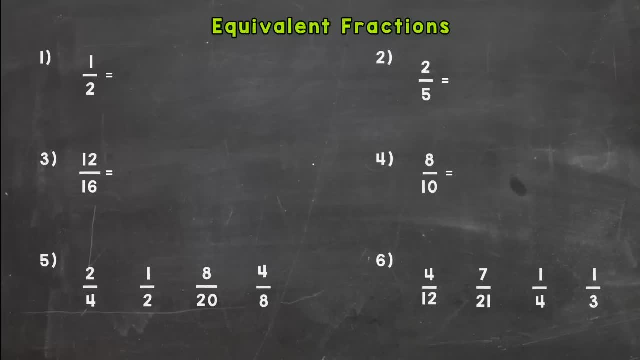 to the denominator, or whatever you do to the denominator, you need to do to the numerator. Now, if you don't know what numerator and denominator are, what those are, those are: the top number is the numerator and the bottom number is the denominator. So whatever you do to the top, 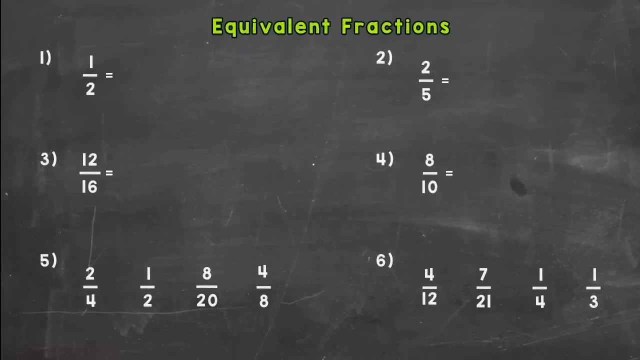 you got to do to the bottom, or whatever you do to the bottom, you have to do to the top and you can use multiplication or division. Now this might be confusing as we first start off, but as we go through, I promise this will get easier and make more sense. And, just like all of my other, 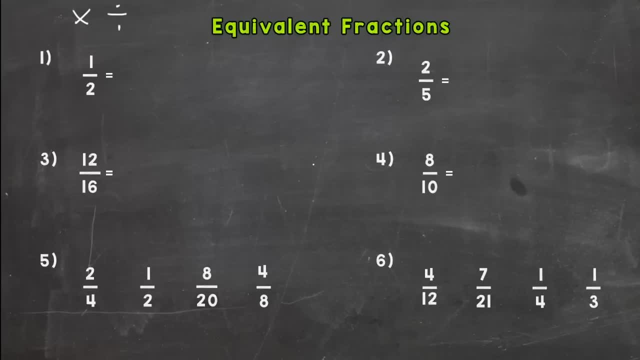 instructional videos. I highly suggest you write these out with me. So let's see one half here. I can multiply those numbers by anything I want, any number in the world, and as long as I do it to both the top and the bottom, the numerator and the denominator, I will. 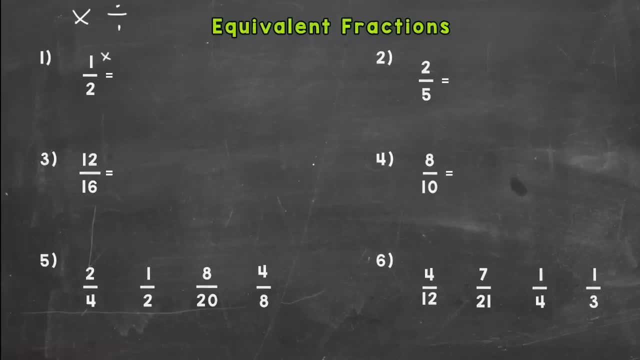 get an equivalent fraction. So let's say I'm going to multiply them both by five and I get one. half is equal to five tenths. Is five out of ten the same thing as a half? Yes, those are equivalent. or maybe I want to multiply them both by two and I get two fourths. 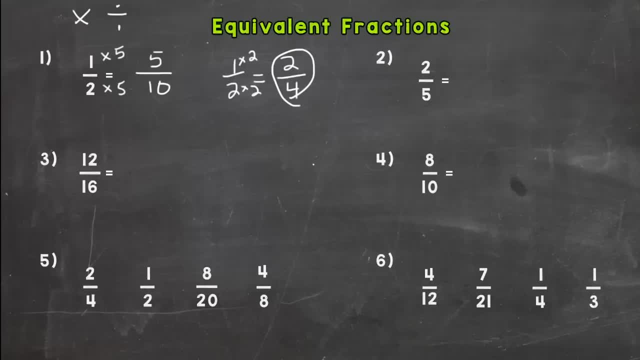 Is two fourths the same as a half. Yes, they're equivalent. So again, as long as I do the same thing to both the top and the bottom, I will get an equivalent fraction. I can use multiplication or division. Now one half if I want, wanted to use division. 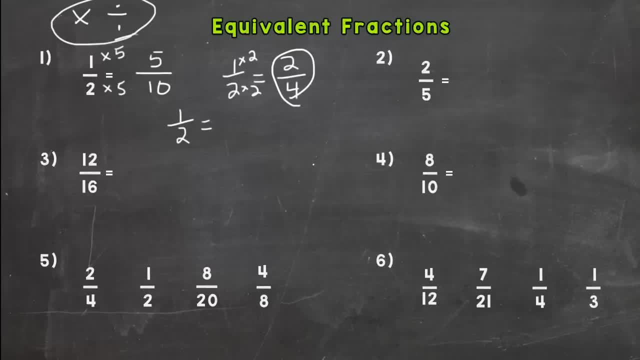 there isn't anything I can divide one and two by. I can't break that down anymore, so I can't use division for that one. And as you do more these you you will see which ones you can use division for and which ones you can't. So that's just something you will get a hang up. get the hang of. 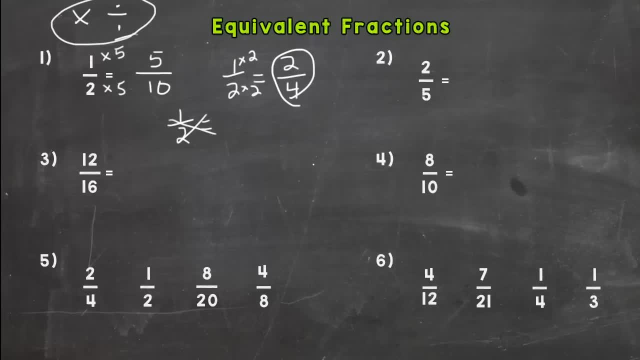 as you do more of them. So number two again: whatever you do to the top, you have to do to the bottom. So I'm going to multiply the numerator and the denominator. So I'm going to multiply the both by 100. And I get 200. five hundredths, That is equivalent to two fifths. And how? 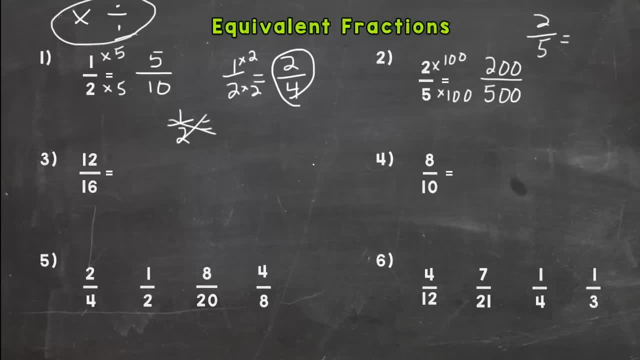 about two fifths. I will multiply them both by three And I will get six fifteenths. Six fifteenths, two hundred five hundredths and two fifths are all of equal value. They just have different names. That's what an equivalent fraction is, If you let's pretend we have. 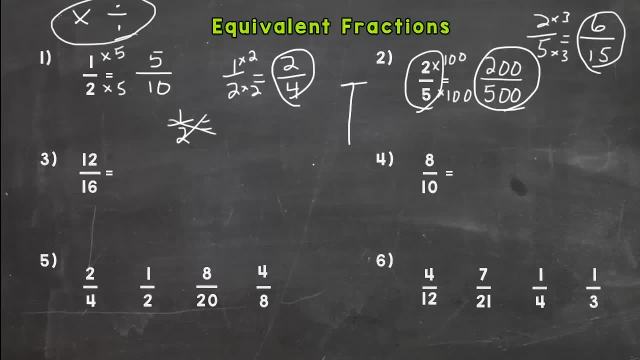 I'm going to draw a terrible scale here, But let's say we're weighing two fractions on each side And we have two fifths over here and two hundred five hundredths over here. They would weigh the same And I'm going to put a base on my scale there. They would weigh. 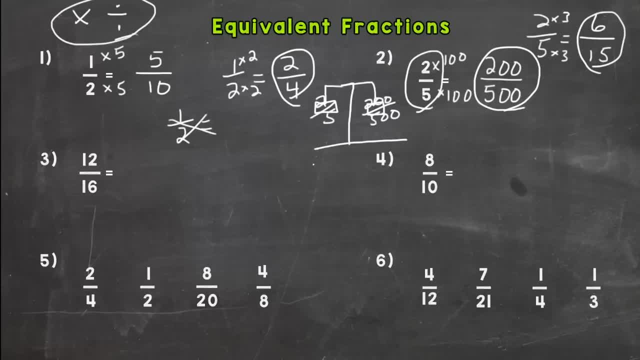 the same. They just have different names, but they are equivalent. We followed our rule: We multiply or divided both the numerator and denominator by the same number. Alright, let's go to number three. We're going to use division on this one, actually for our first. 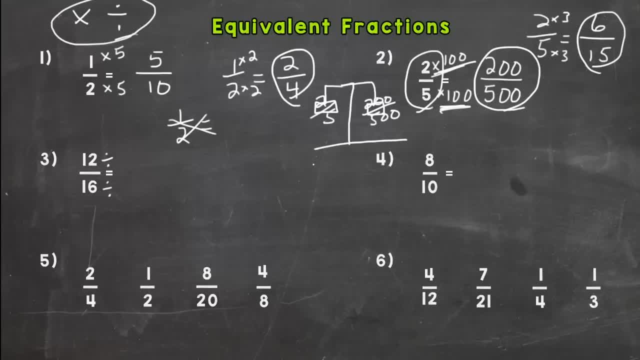 equivalent fraction. What can twelve and sixteen both be divided by? Well, they're both even. so what goes into all even numbers? I'm going to divide them both by two to get an equivalent fraction, Six, eights, And then I will use another division, one actually. 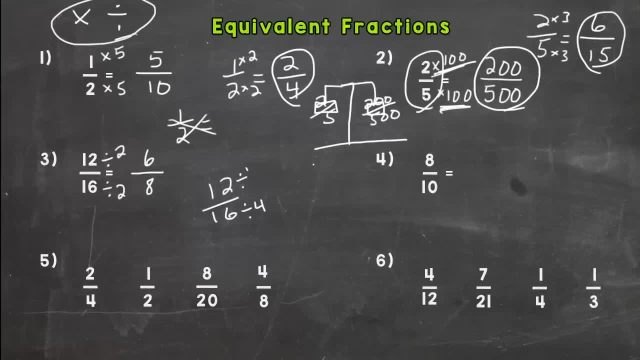 Let's see who is really on the ball here. I gave it away though Four. I can divide each of those by four. That's a common factor or a common number that can be divided out of both twelve and sixteen. So twelve divided by four is three. 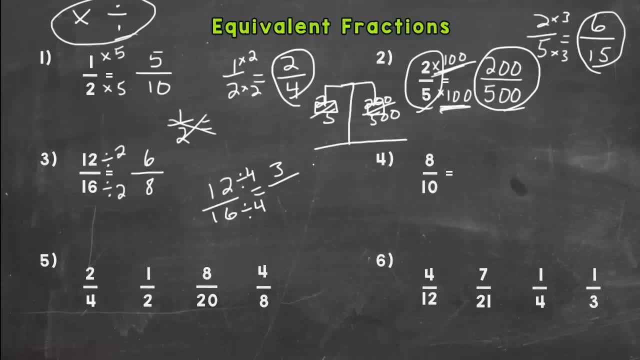 Sixteen is nine And twelve is thirty, Sixteen is five, Sixteen is seven, Seventy-eight, eighty and eighteen. 16 divided by 4 is 4.. Since I gave that one away, let's try division for 8 tenths. 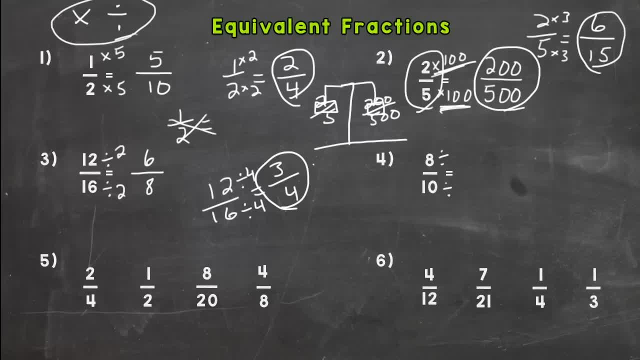 Think to yourself: what can I divide both 8 and 10 by to get an equivalent fraction? Well, they're both even. There's your hint. Hopefully you're thinking 2.. I can divide both of them by 2 to get an equivalent fraction, and I get 4 fifths. 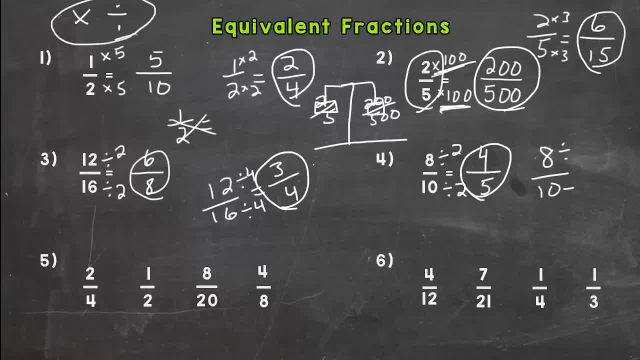 And then let's use a multiplication. Let's multiply them both by- oops, that's a division sign. I said multiply, Multiply them both by 3, and I get 24 thirtieths. So that's how you find equivalent fractions. 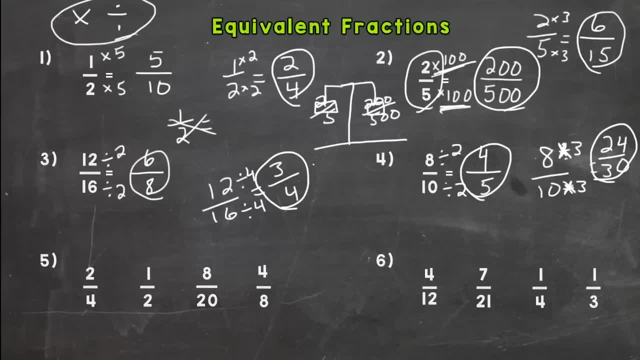 Follow that main rule: Use multiplication or division, and whatever you do to the top, you have to do to the bottom. So let's go to number 5 here And we have 4 fractions. This is kind of like equivalent fraction. I spy, I guess you could say. 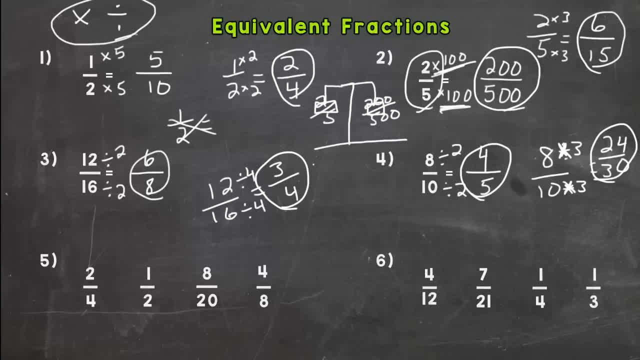 You are finding the fraction that does not fit in the list. There are 3 that are equivalent and 1 that is not. I'll give you a hint for number 5.. We want to find the one that is not equivalent to 1 half. 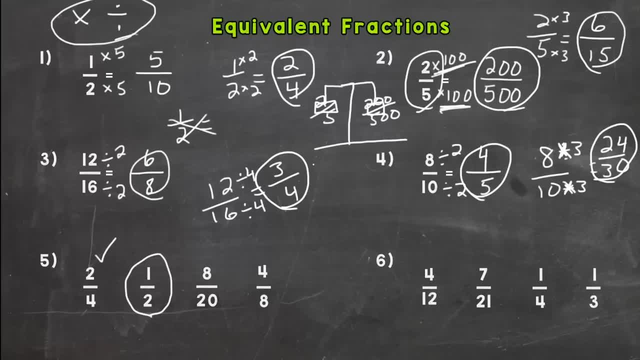 So 2 out of 4 is a half. right. I can multiply The top and the bottom by 2 to get 2 fourths. 4 out of 8 is a half. I can multiply the 1 by 4 and the 2 by 4.. 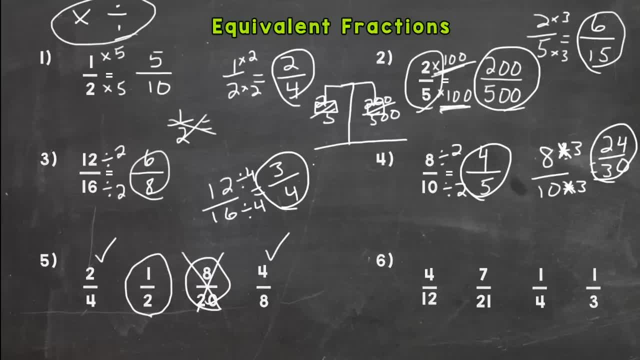 8 out of 20 is the one that does not fit. That is not equivalent to 1 half, So that would be your answer. 8 twentieths is the one that doesn't fit. So let's go to number 6, and I'll give you a hint here.